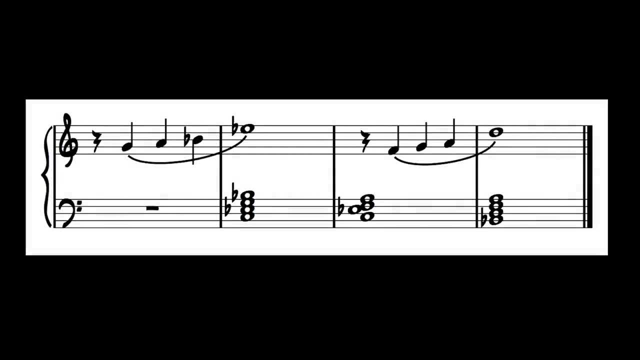 the music, how the notes are spaced out and all of that. So in my opinion, if you're just interested in learning the basics of reading music, then don't worry about rhythm. Rhythm is what takes a lot of time to learn. That's what intimidates most people from learning to read music. 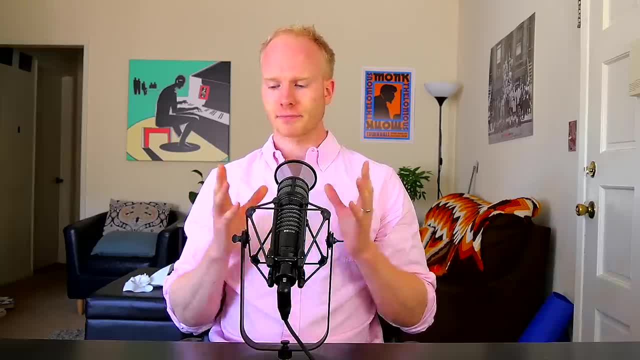 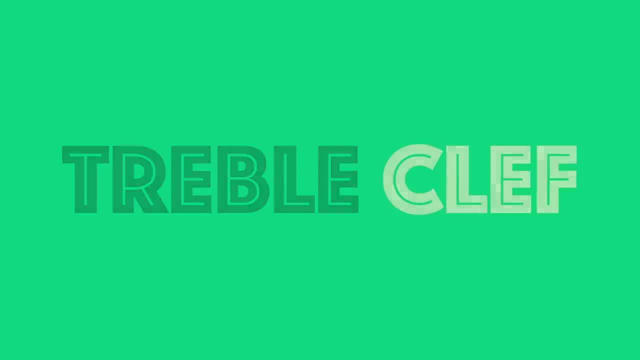 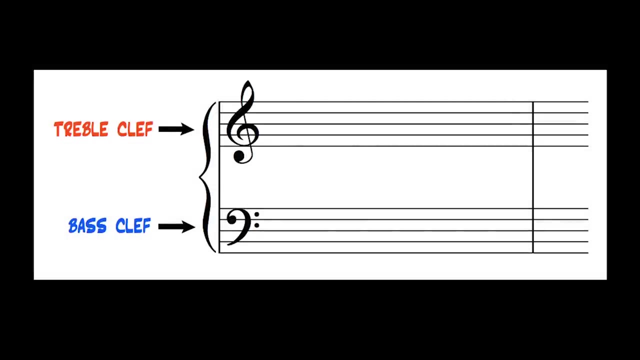 and in my opinion it's not that important. So there are different types of clef. There are two main types of clef, which are treble clef and bass clef. You could think of treble clef as the right hand on the piano- it's the upper part- and bass clef as the left hand on the piano. 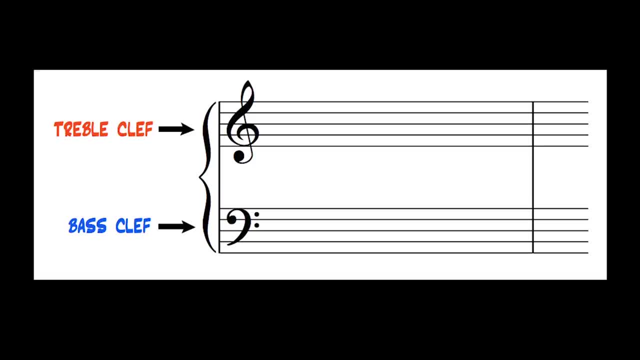 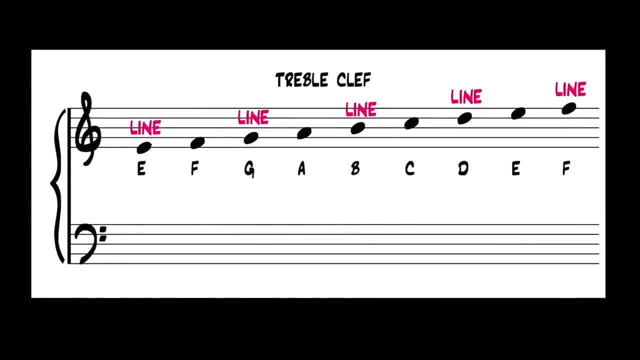 it's the lower part. Now, the way music works with any stave is the lines and the spaces are each their own note. So to move up a note, you go from a line to a space, to a line to a space, The space. 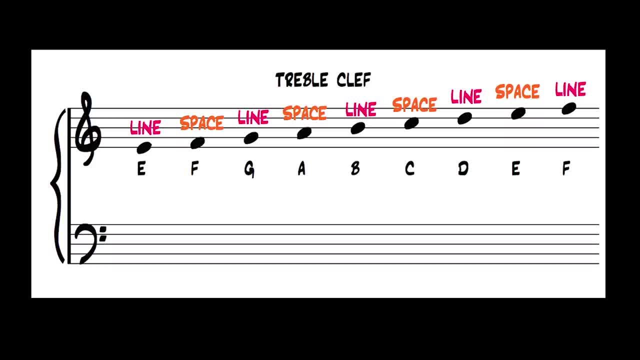 means the space between the two lines. So with the treble clef the bottom line is an E, and then the bottom space is an F, And then the treble clef is an E, and then the bottom space is an F, And then the 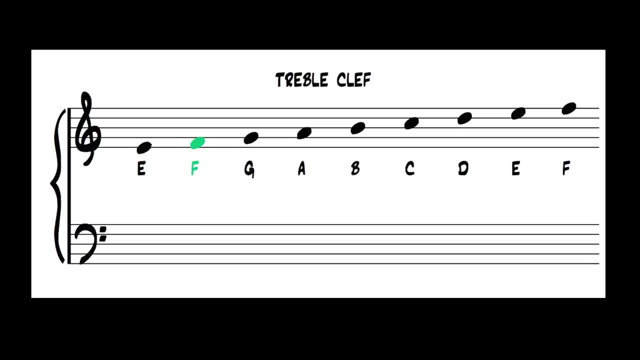 second line is a G, the second space is an A and then it just goes up from there. So B, C, D, E and F. Now the easy way to identify notes quickly is to use an acronym to remember the five lines. 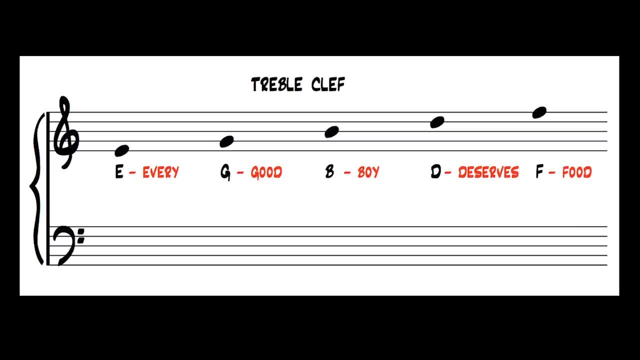 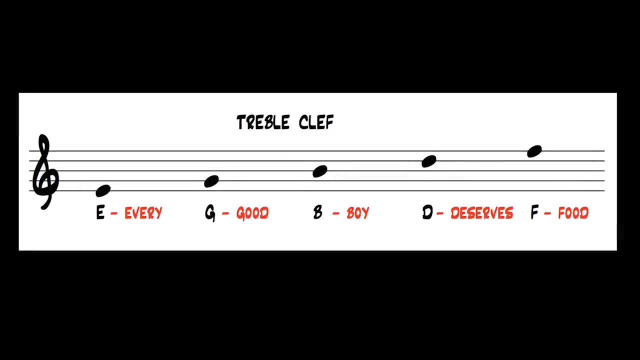 So the common one that I was always taught is: every good boy deserves food And really catchy, I know, but it's stuck And that's what I've always used. And if you have your own acronym that you use, please post it in the comments below. So every for E, good for G, boy for B. 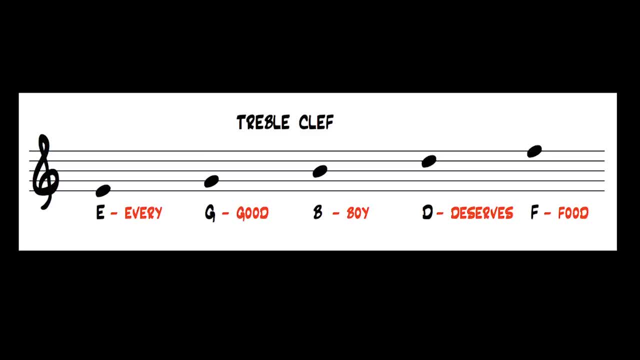 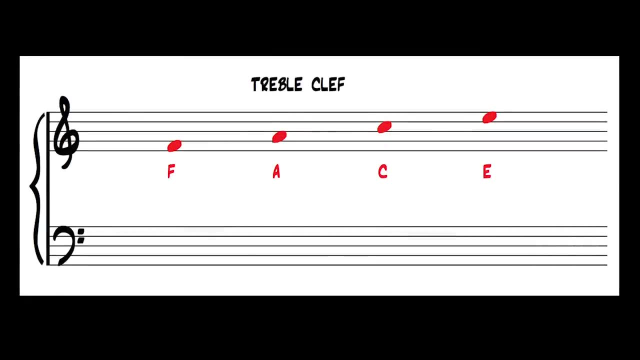 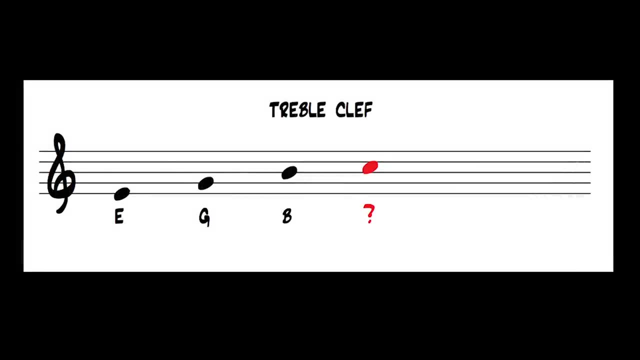 deserves for D and food for F. And then some people like to do the same for the spaces and they'll use the word face, which is what the spaces spell out. But if you like, you can just use the lines to remember the spaces. So, for example, we have E, G, B, well, B plus one. 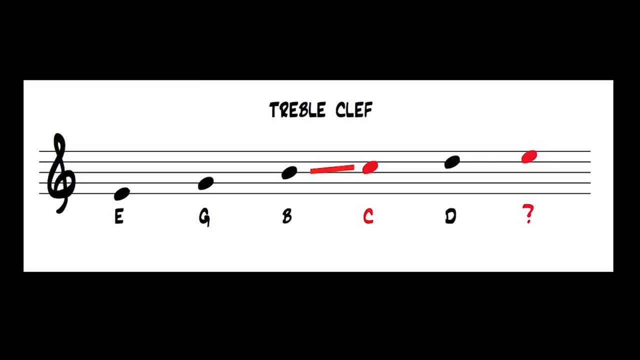 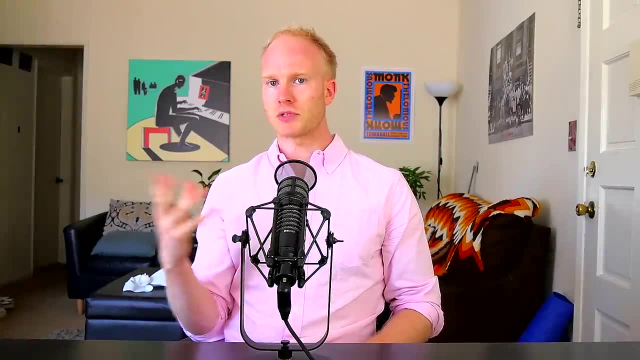 is going to be C or D, plus one is going to be E. Now, the other thing to mention is that these aren't just any old E, not just any old G, any old B. These are actually specific notes within a specific octave. 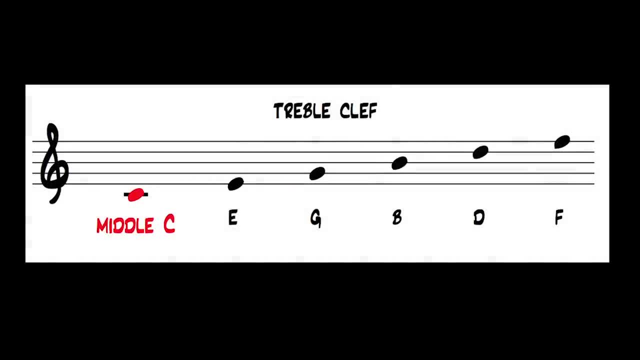 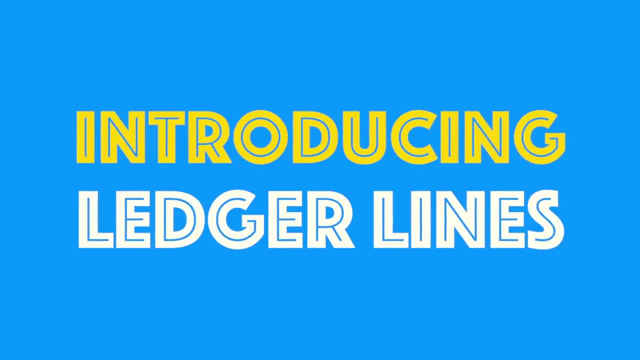 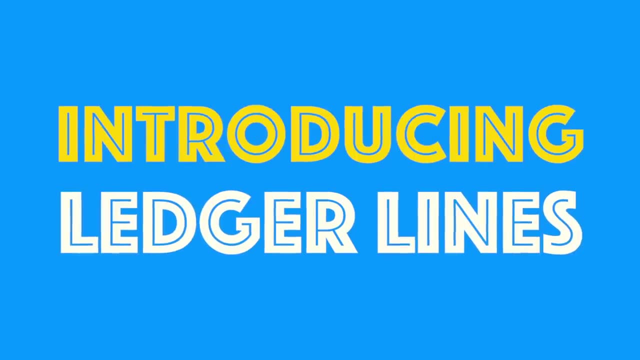 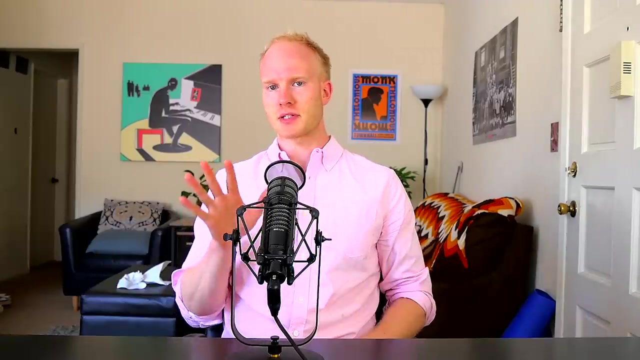 So with the treble clef the bottom E is specifically the E above middle C on the piano. Now it's also possible for these notes to go above and below the stave. so there's just five lines, but obviously these notes can go above those notes. 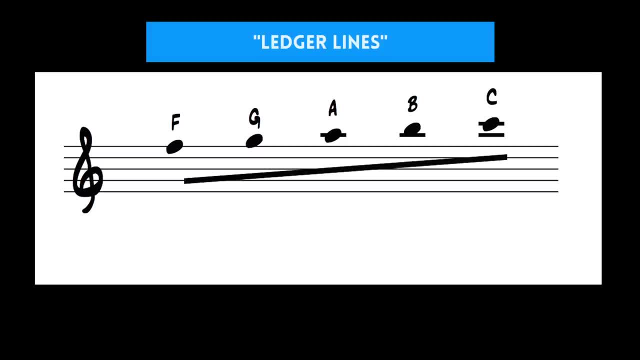 And when this happens we use what's called ledger lines, and these are pretty logical. They're basically just lines which get added to that note so that you can measure up beyond the top F and below the bottom E. And it gets a bit tricky sometimes to read these ledger. 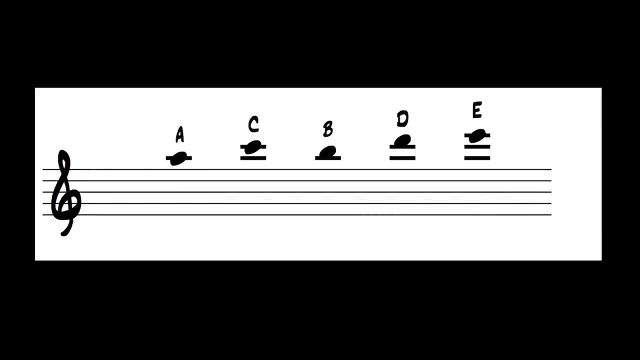 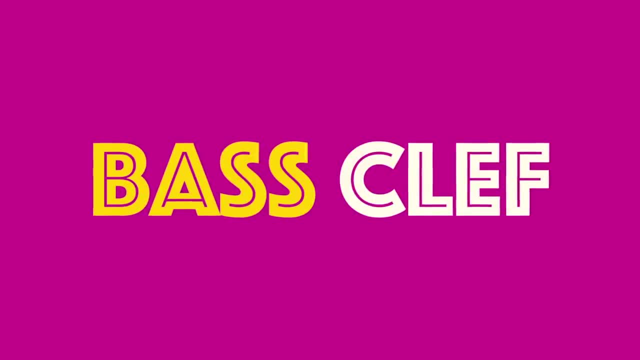 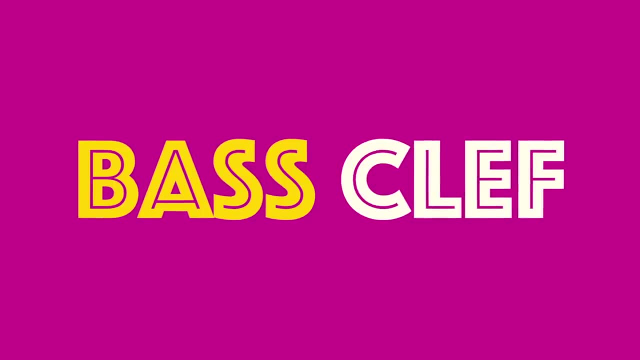 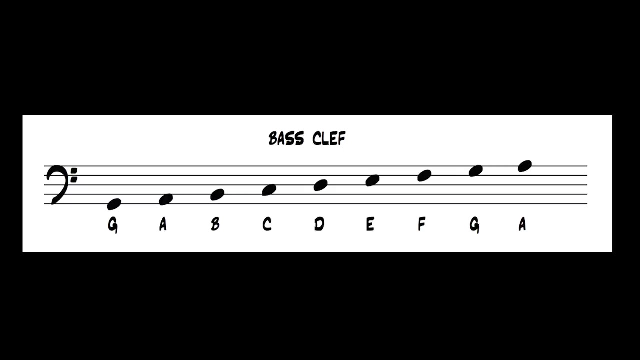 lines, because you're not often looking at them. But sometimes you have to sort of count up literally every single note, and that's fine, that's natural. So next up, we have the bass clef. Now with the bass clef, unfortunately we don't have 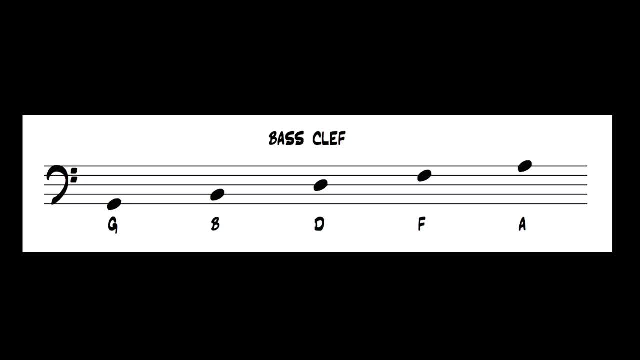 the same letters, Although it could very nearly be the same as E, G, B, D, F. It's a bit of a shame We actually have to learn a new acronym to remember this one. I guess it's not an acronym, a rhyme though. 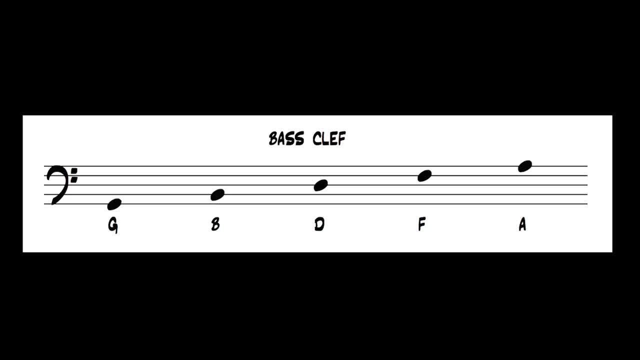 to remember the lines. So with the bass clef the lines go G, B, D, F and A. Some people use Good Boys, Deserve Fine Apples. Some people use Grizzly Bears- Don't Fear Anything, And in fact I actually prefer the ones that don't have. 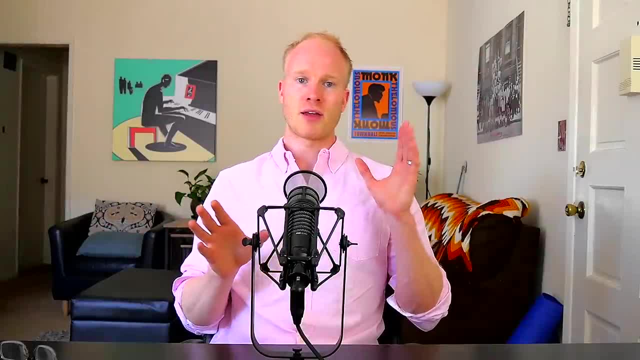 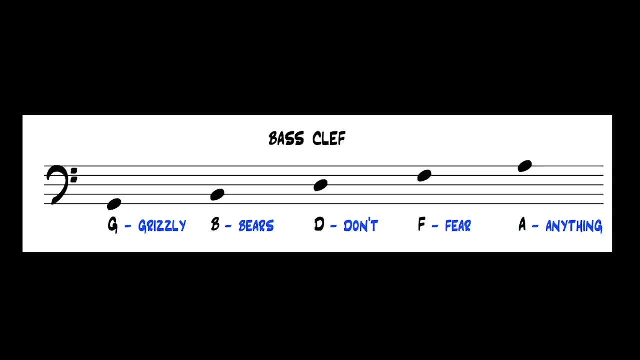 Good Boys Deserve, because you can get confused with the treble clef and the bass clef since they're both very similar. So I would use Grizzly Bears. Don't Fear Anything, because there's less likely that you'll get confused. 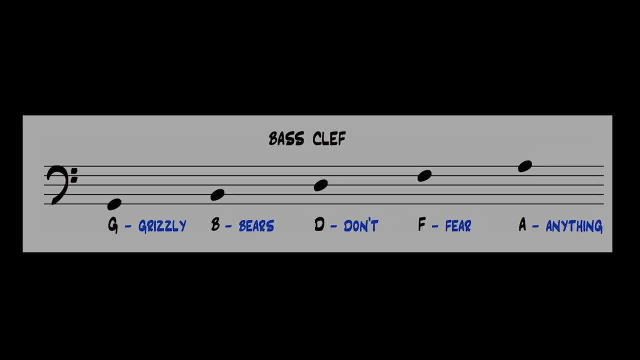 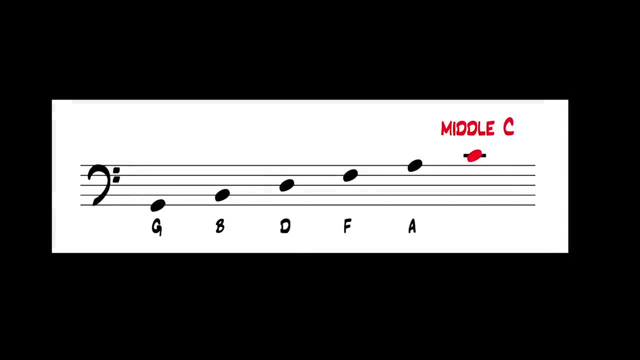 with the treble clef. Now it's also important to know where on the keyboard these five notes are: G, B, D, F, A. So the way to remember the register is that middle C is one ledger line above the top left. 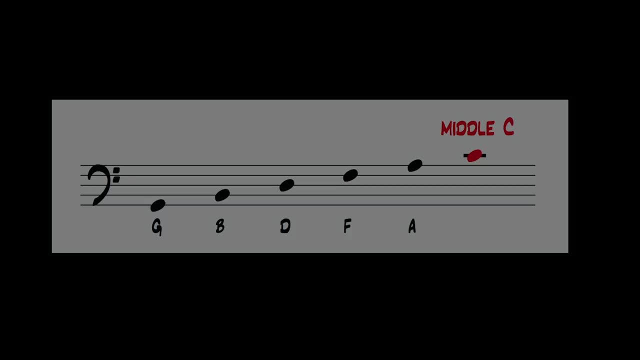 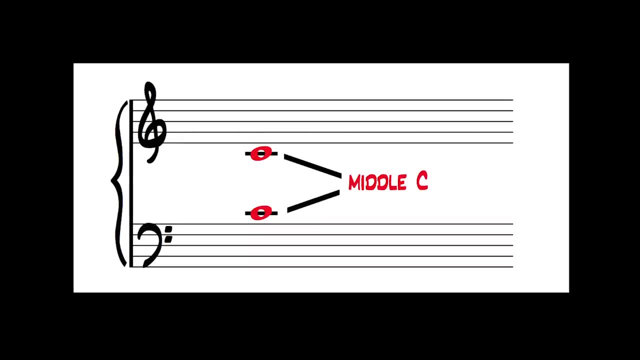 And middle C is one ledger line above the top left And middle C is one ledger line above the top left. So this is actually a good way that you can remember both the treble clef and the bass clef. They're actually sort of like a mirror of each other. 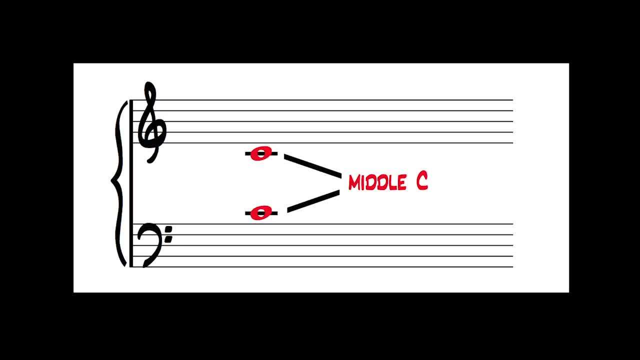 because on the treble clef, middle C is one ledger line below the bottom line, And then with the bass clef, middle C is one ledger line above the top line. So if you take nothing else from this lesson, you can just remember where middle C is. 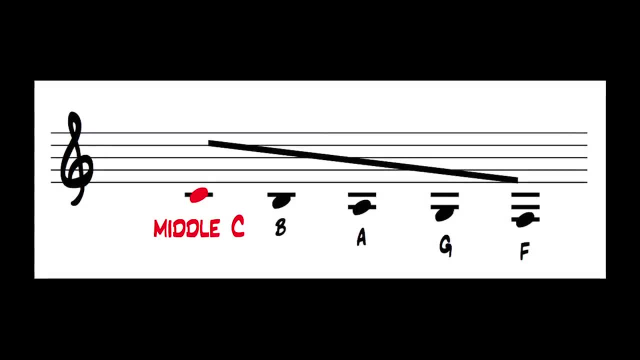 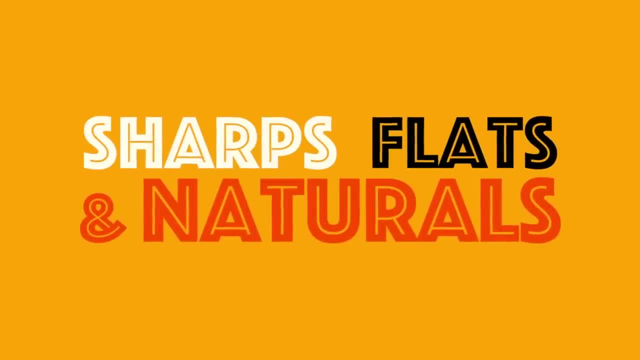 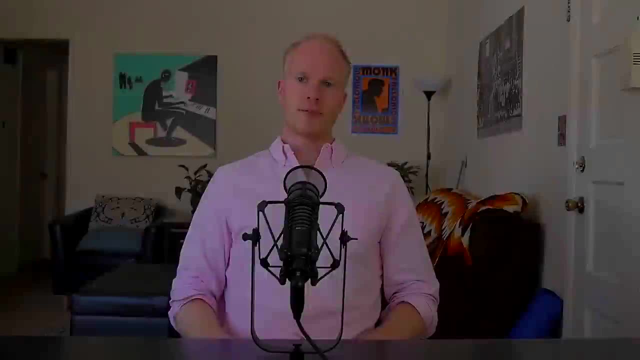 You can count up or count down and figure out any note, So it might take you some time, but that's certainly something you can do as a last resort method. Now in music any of these notes can be sharpened, which means raised a half step. 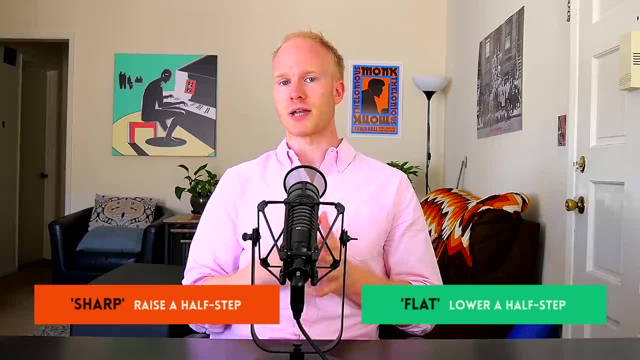 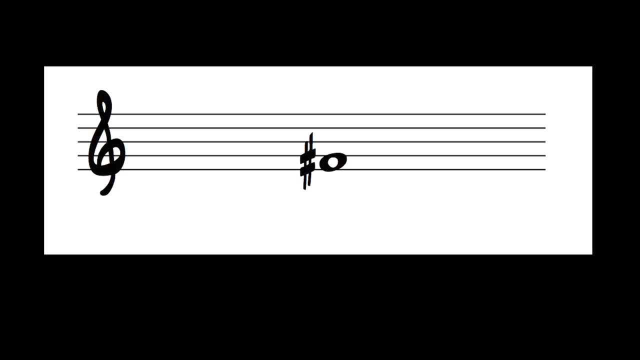 And any of these notes can be flattened, which means they're lowered a half step. Now, the way that we write a sharp, we're going to do this, So you'll see this little sign. It's basically the pound sign on a phone. 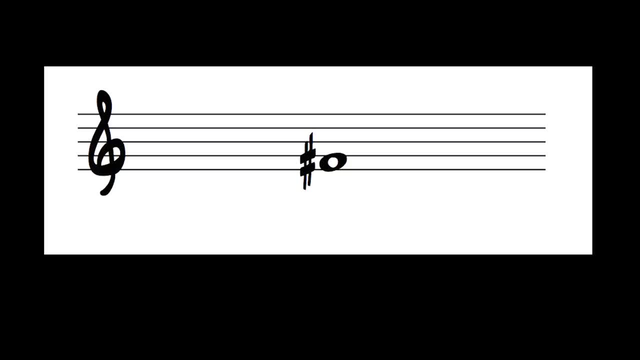 And it will appear just before the note which is to be sharpened. So see if you can tell me which note we're looking at here. Well, it's the lowest space in the treble clef, which means it is- that's right- an F. 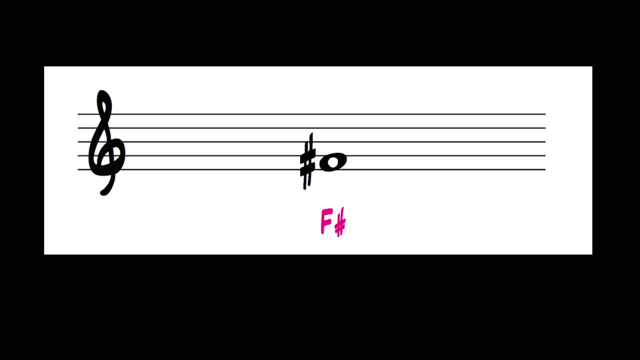 And there's a sharp sign in front of it which means it's an F sharp. And we have this sign basically like a tiny B and it goes just in front of the note which is to be flattened. So let's see if you can work out which note this is. 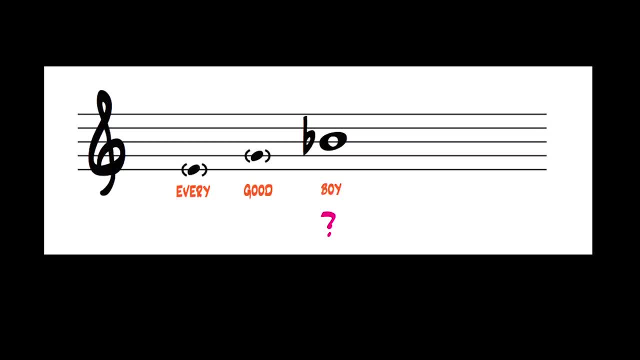 So it's treble clef. We'll use the rhyme every good boy. So it's a B and there's a flat sign in front of it, which means it's a B flat. Now once a sharp or a flat sign. 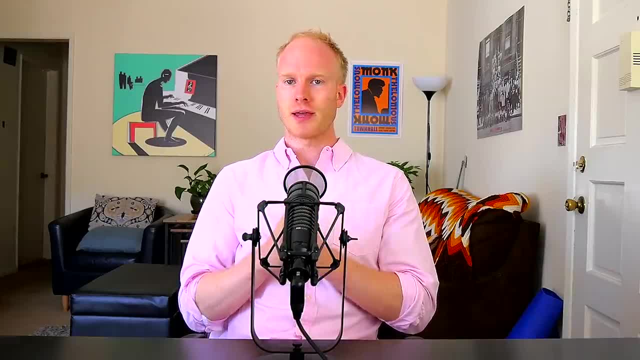 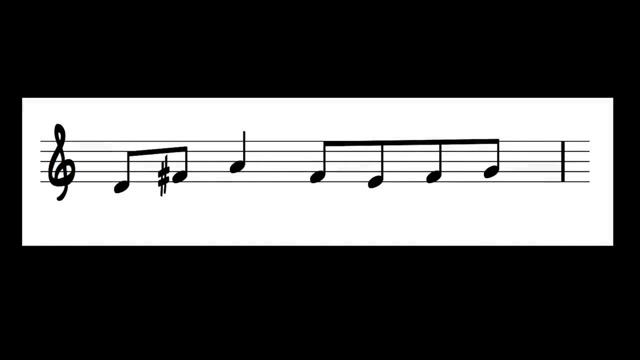 has been used, it doesn't just affect that one note, It also affects any repeats of that note for the rest of that bar. So if there was another F or another two or three Fs played after that F sharp, well, they will all be made F sharps. 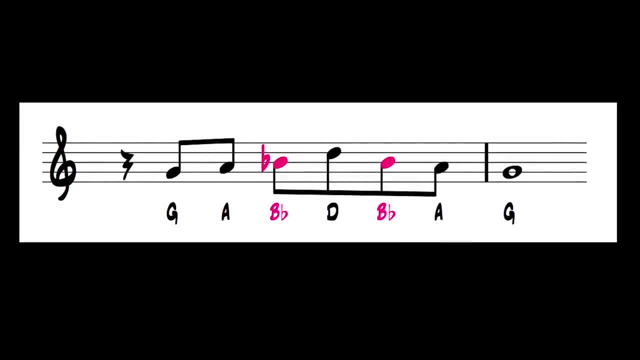 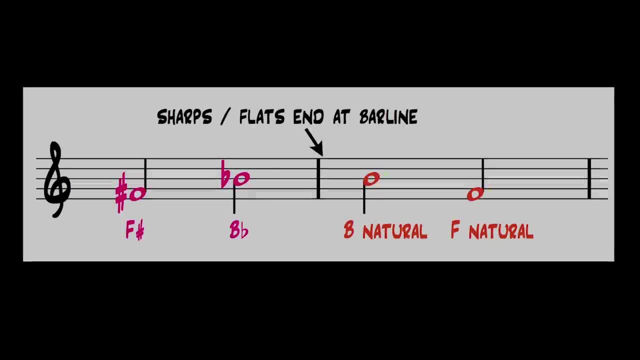 Or if there's another B after that B flat, well that will also be played as a B flat as well. And then, once you get to the next bar, you'll get a bar line, which is a vertical line. then it resets. 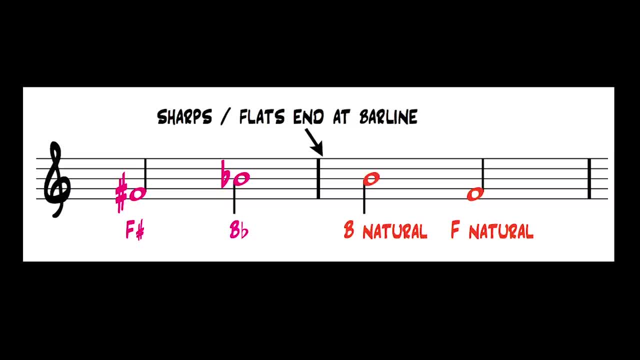 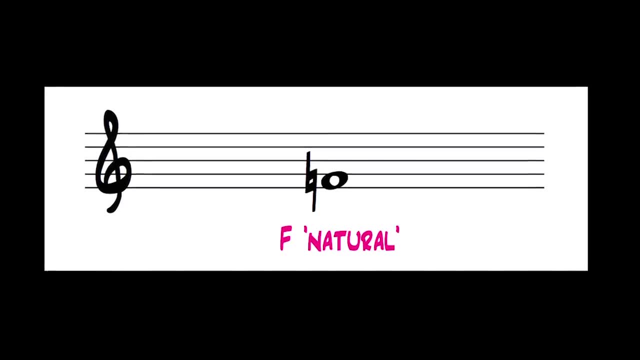 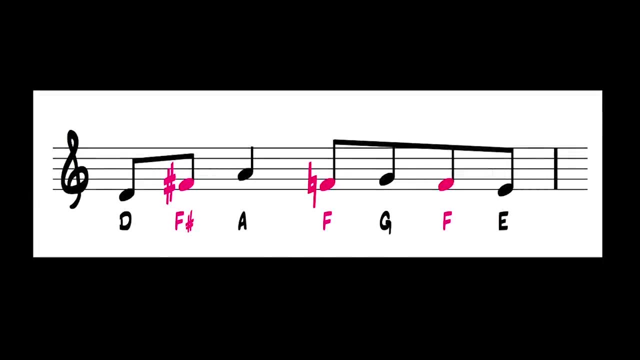 And then any Bs or Fs will be B naturals after that. Now there's also a natural sign which looks like this, And this symbol basically undoes the effect of the sharp or the flat from earlier in the bar. So say you had the F sharp. 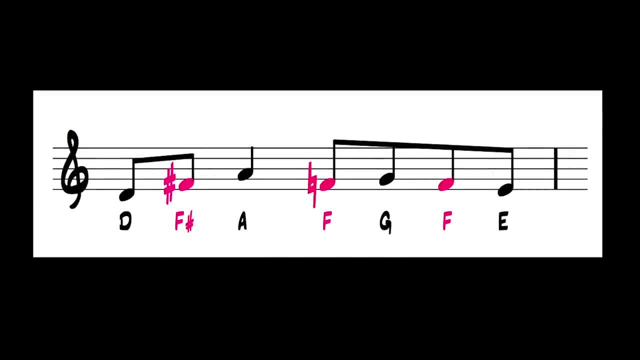 but then on the repeat of the F sharp it'll actually have this natural sign just before it. That would mean it's back to F natural again. And then if there were any repeats of that F- F in the rest of the bar it would be played a natural. 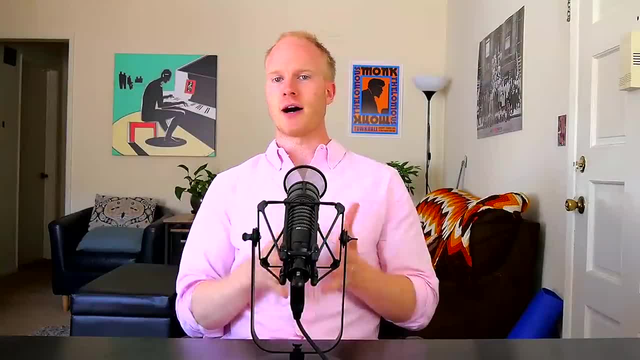 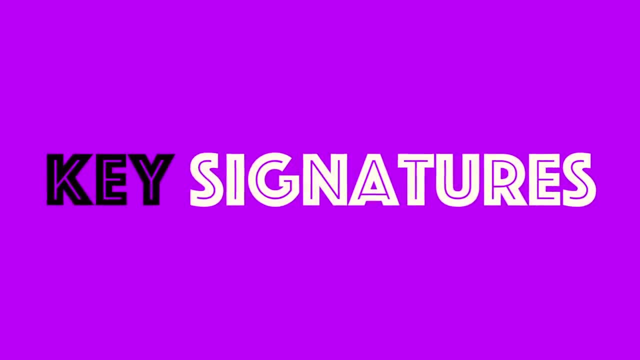 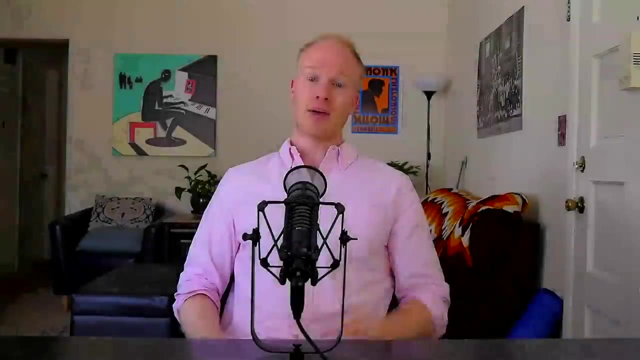 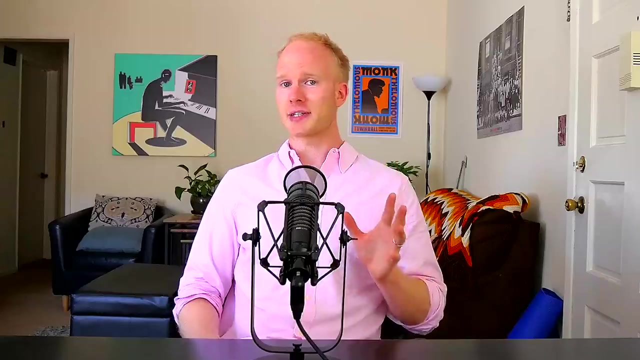 So this natural also gets used and it's basically a way to undo the effect of the sharp or the flat. And one final point to make on sharps and flats is at the very beginning of the piece you might have what's called a key signature. 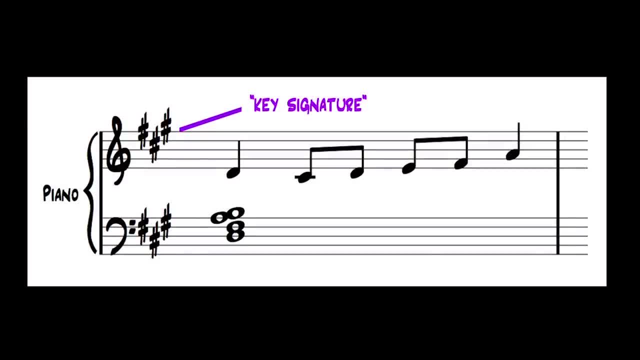 Key signature is basically a display of sharps or flats. So you might have say F sharp and C sharp at the very beginning of the piece, before the music even starts. It basically means that this will be valid throughout the piece. So every time you see an F, it's gonna be an F sharp. 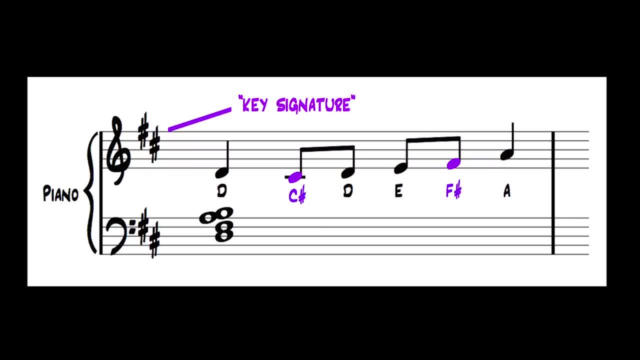 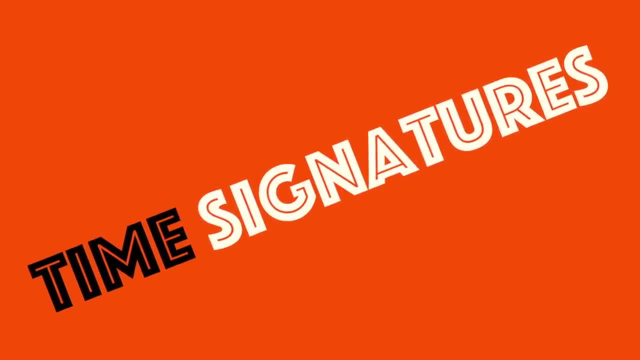 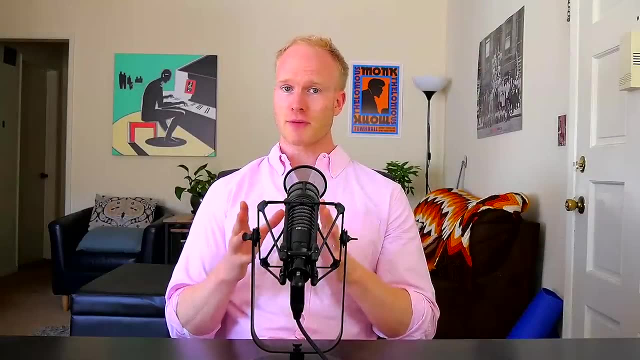 Every time you see a C, it's gonna be a C sharp Now. at the beginning of the video, I said I wasn't gonna cover rhythm. However, there is one thing I just wanna say on rhythm, and that's about time signatures. 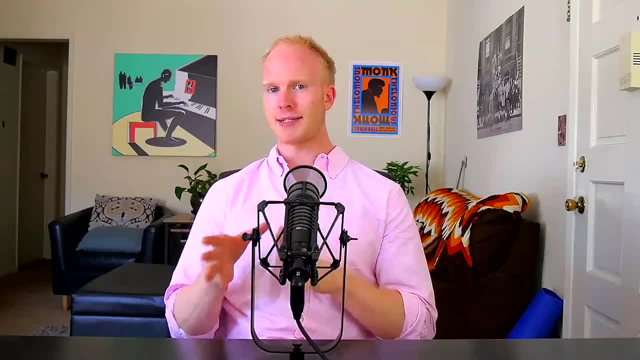 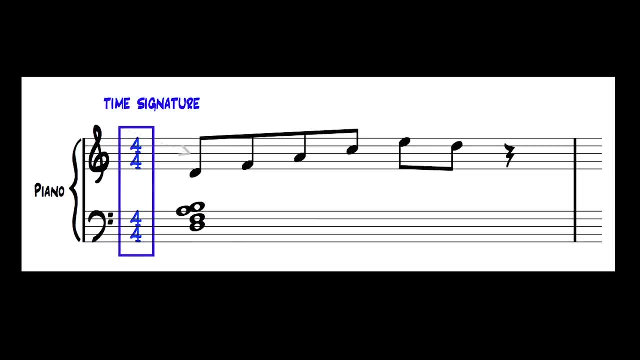 So if you look at the beginning of the piece of music, just as I said, there's a key signature. You'll also see a couple of numbers on top of each other, and this is what's called the time signature. Now, these two numbers tell you what type of time signature. 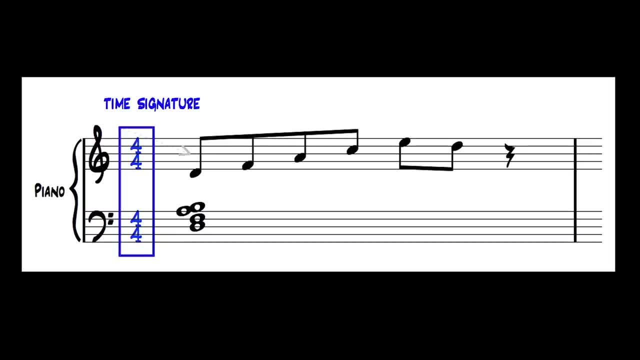 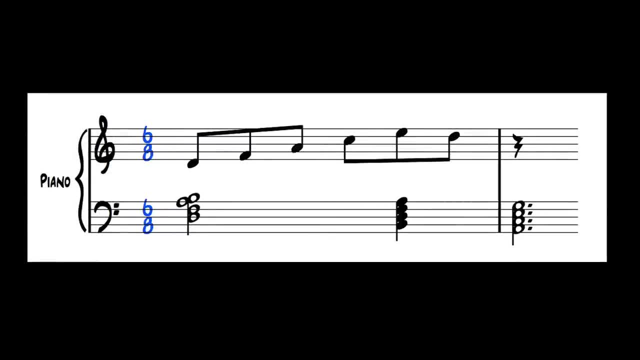 It could be three-four, It could be six-eight, It could be seven-eight, five-eight, all these different time signatures. Now the important number is the top number, So it tells you how many beats are in the bar. So if you see four-four, 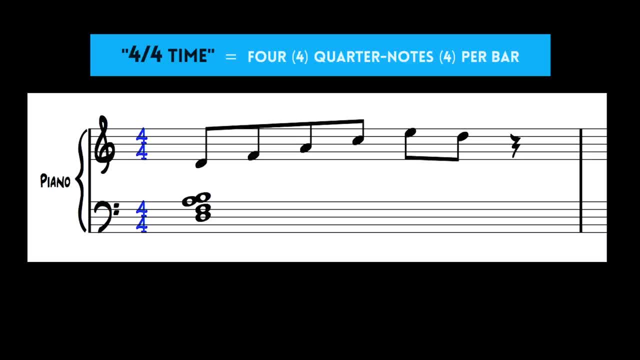 that means there are four beats in the bar: One, two, three, four. One, two, three, four. One two, three, four. If it's three-four, that means there are three beats in the bar: One, two, three. 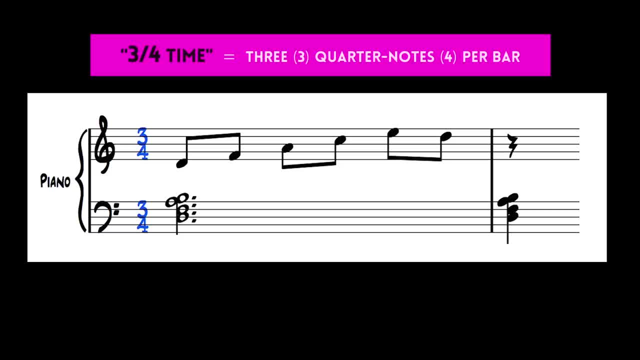 One, two, three. One, two, three, which has more of a waltz feel. For example, if it is six-eight then it has a sort of swing type of feel. One, two, three, four, five, six. 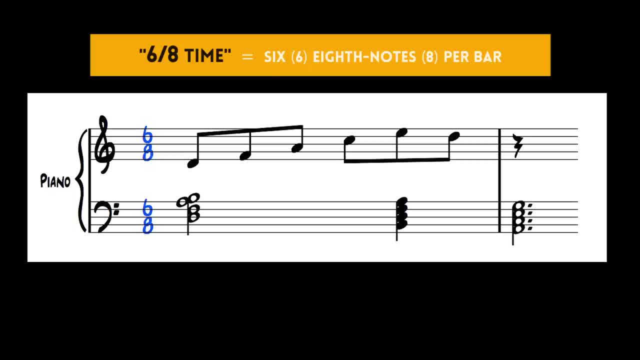 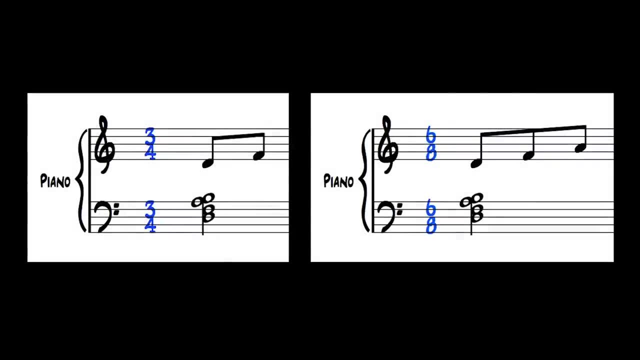 One, two, three, four, five, six. One, two, three, four, five, six, And so on. And then the bottom note is less important. It tells you what type of beat that is, But it's not too important whether it's a four. 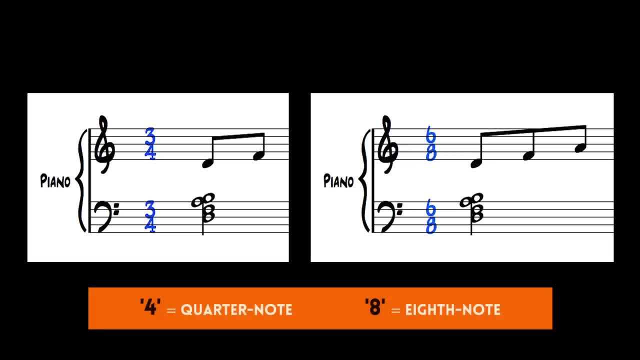 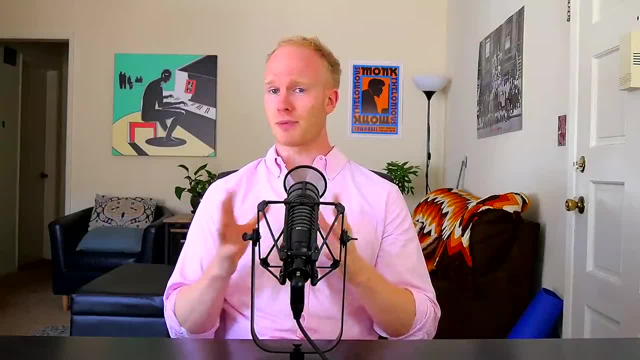 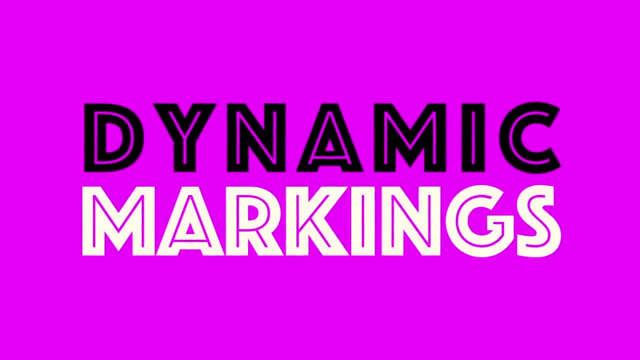 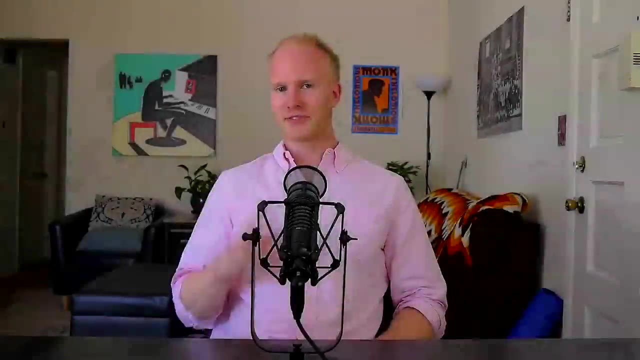 or it's an eight. Usually it's one of those two, So that can also be useful to understand what those two numbers at the beginning of the music are. Well, it's the time signature. So finally, I'm just gonna go over. 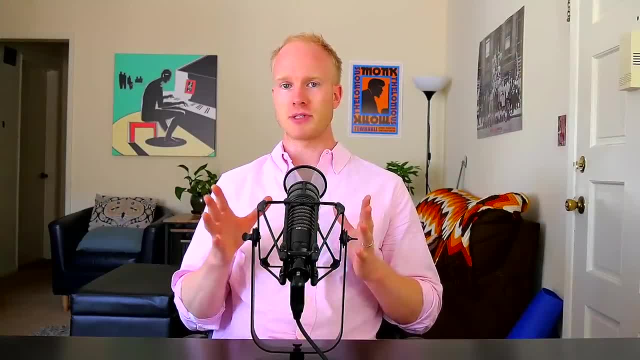 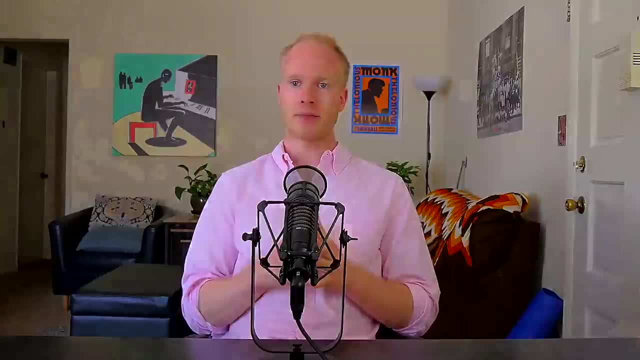 a few remaining notation markings which you'll also encounter in music. First up, we have dynamics. What are dynamics? Well, it means how loud or soft you want to play. So generally, you have P and you have F, So you'll see these Fs and these Ps. 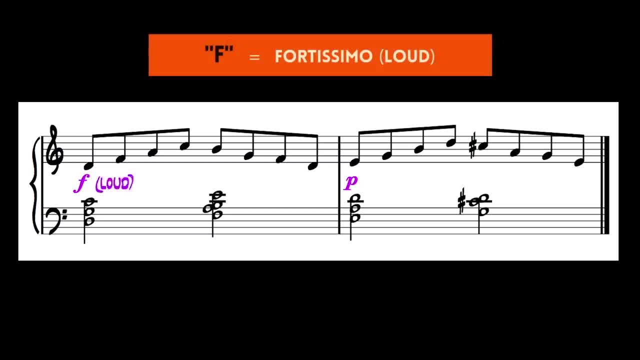 scattered about the music. F stands for fortissimo, and it means play it loud, And P stands for piano, which means play it quietly. Now, sometimes composers will stack up the Fs, which means basically: the more Fs, the louder. 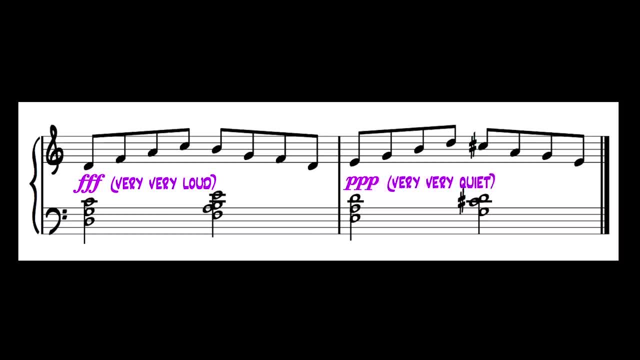 Same with the Ps goes down to about triple P. It's pretty rare to see anything beyond that. You'll also get MF and MP. You'll also get MF and MP. You'll also get MF and MP, And that just means mezzo forte or mezzo piano. 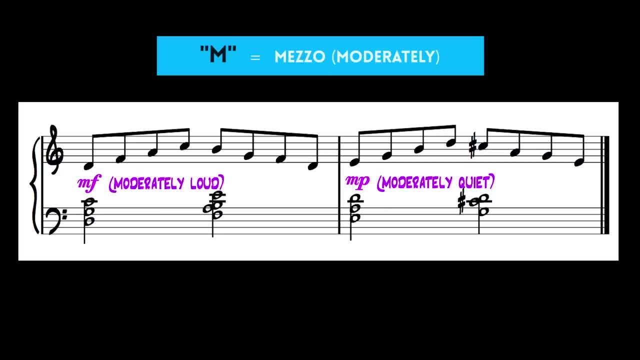 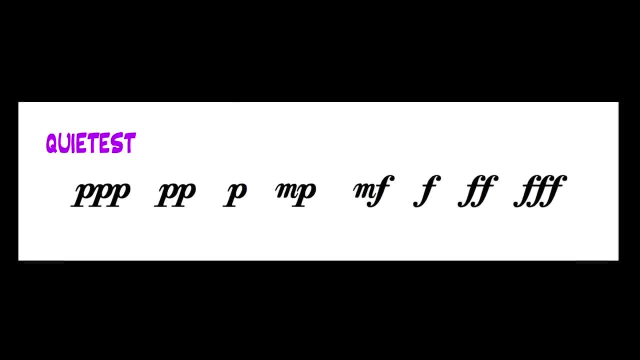 Mezzo basically means medium, So you'll have medium loud and medium quiet. So if we just take a look at this diagram, you'll basically see from the far left you have the quietest, going through to the far right where you have the loudest. 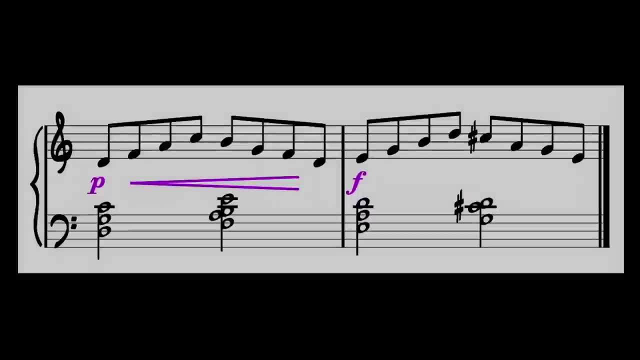 And another dynamic marking you'll also see is these sorts of hairpin notation. So when the hairpin expands to the right, this is called a crescendo, It means get louder. And then when a hairpin gets smaller to the right, that's a diminuendo, and that means get quieter. 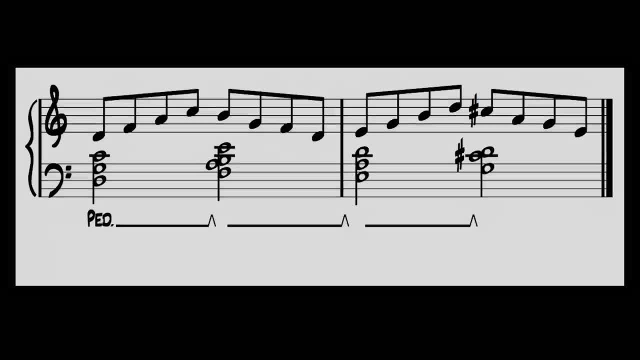 Now, if you're a piano player, you'll also encounter pedal markings. Basically, you'll see a sustained light and quiet sustained line below the stave. As long as that line is sustained, it means hold down the pedal. 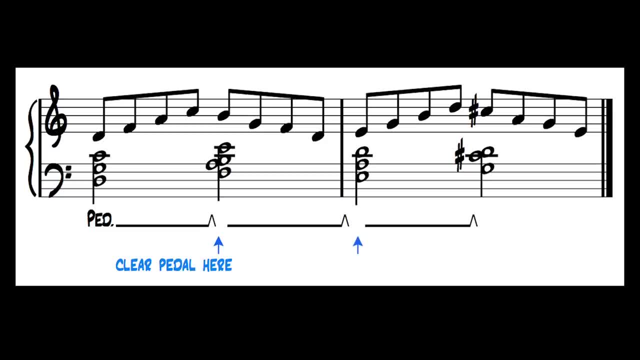 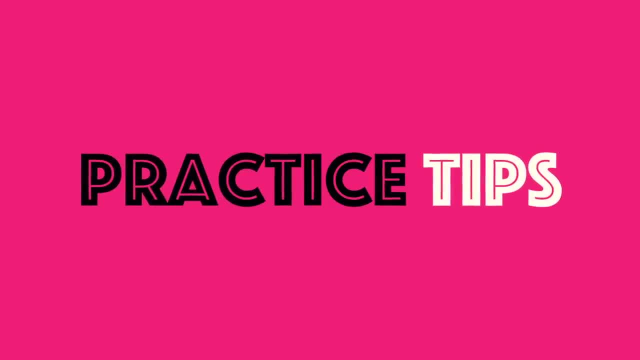 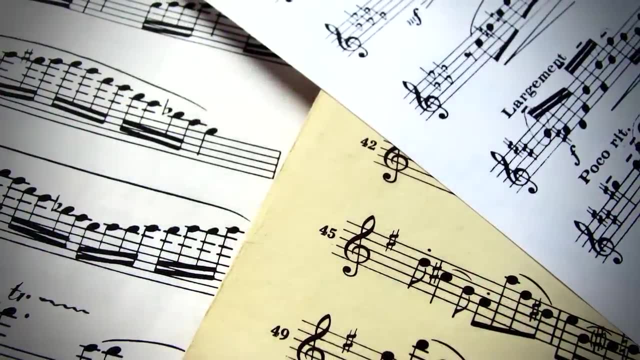 And then when there's a break in it, it means clear the pedal and then it'll start again. Now, finally, you'll want to practice this. It'll probably take a couple of weeks to ingrain everything which I've just shown you. 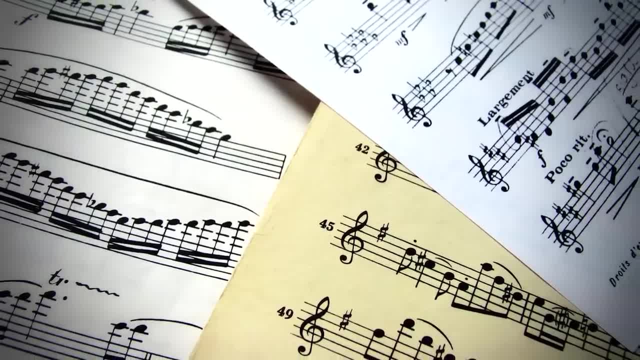 Now there are two ways to practice reading music. The first is to focus on the piano. The second is to focus on the piano. The third is to find some sheet music and practice sight reading. Now I'll put a link below this video. 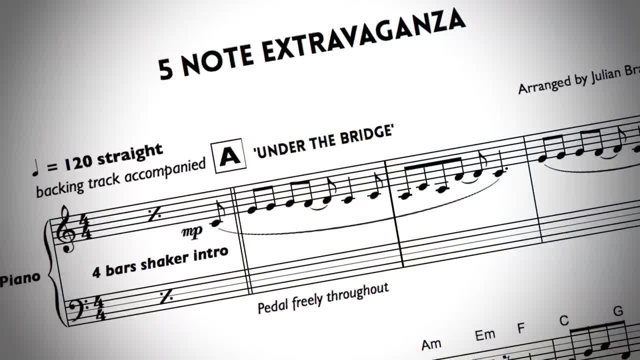 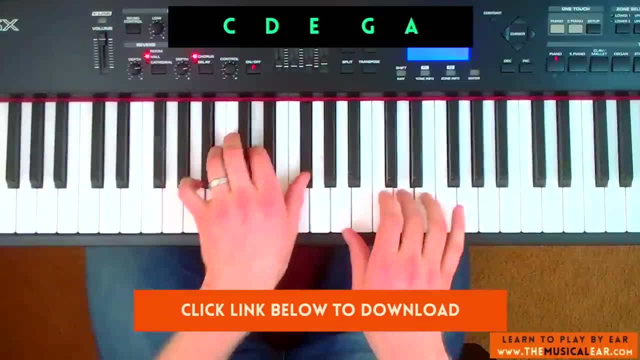 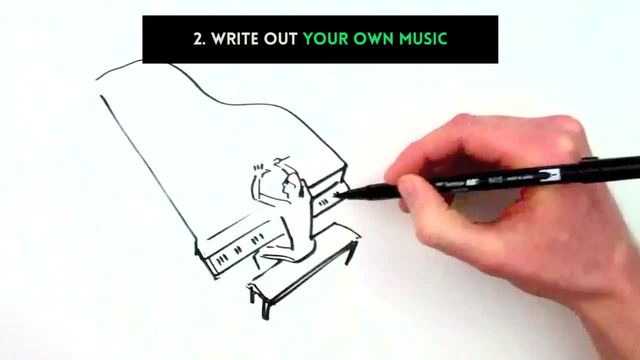 to some of my free sheet music. There's my five-note extravaganza piece, which was a medley I posted recently. It comes with a backing track, And the second way is to practice notating your own compositions, So maybe you have a piece of music you play. 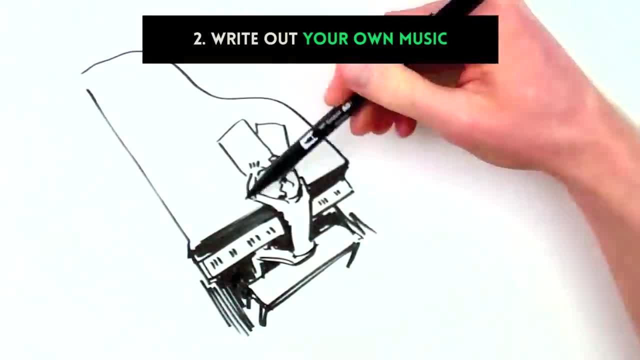 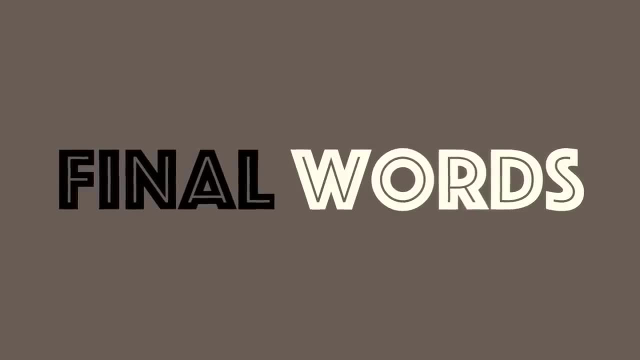 Well, practice finding the notes and writing them out on the stave. And if you have a piece of music you want to practice, you can do that on the stave, And then you can play it on the stave. And then you can play it on the stave. And then you can play it on the stave. 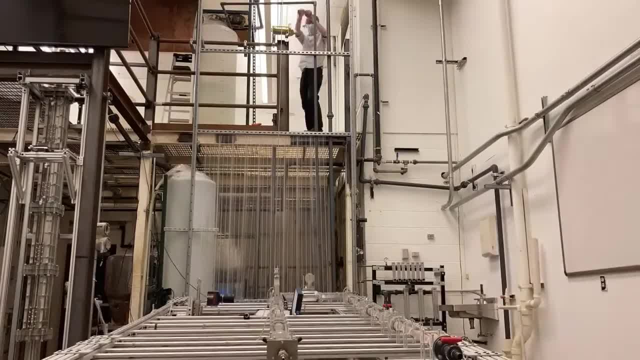 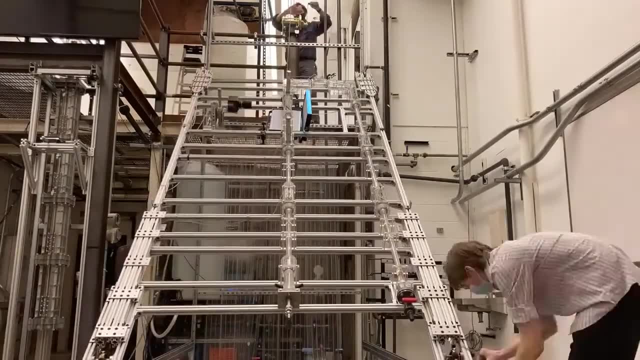 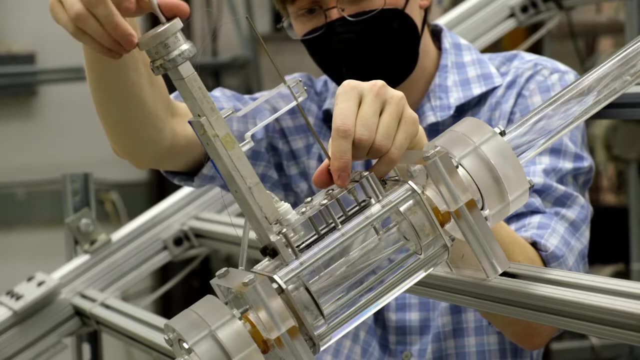 Most two-phase flow experiments have been vertical and little work has been done for other angles. This inclined touch facility is capable of investigating a full range of angles for upward and downward two-phase flows. Local data is collected using state-of-the-art conductivity probes. The signals from these sensors can be used to calculate the time.